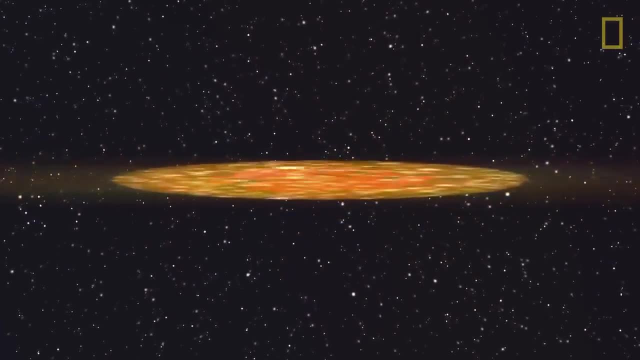 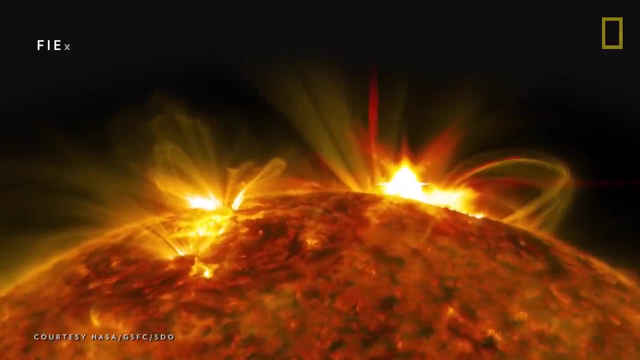 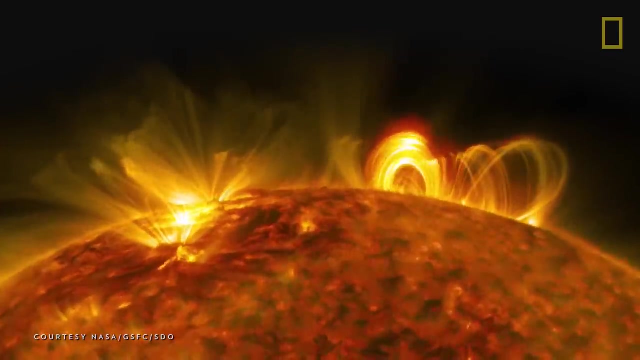 known as a solar nebula, collapsed, And in the middle of this formation, water condensed into a burning ball of gas that became our Sun. The Sun's fiery nature, along with a tremendous gravitational pull and an extensive magnetic field, helped it to become the heart of our solar system. 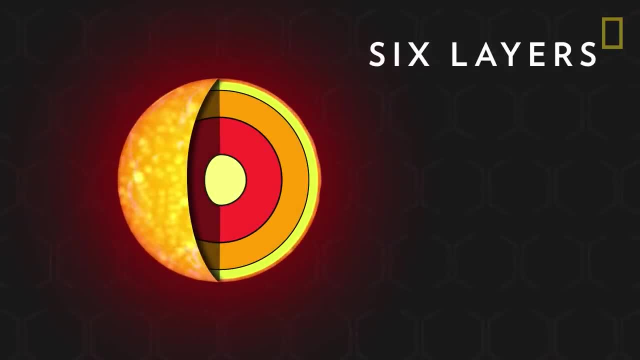 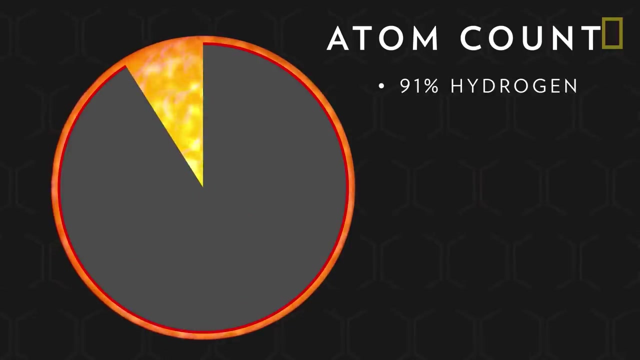 The Sun can be divided into six layers or regions: The corona, the chromosphere, the photosphere, the convective and radiative zones and the core. In terms of atom count, the Sun is about 91% hydrogen, the Sun's fuel. 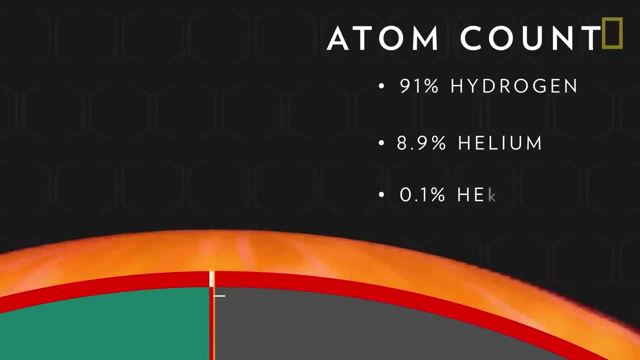 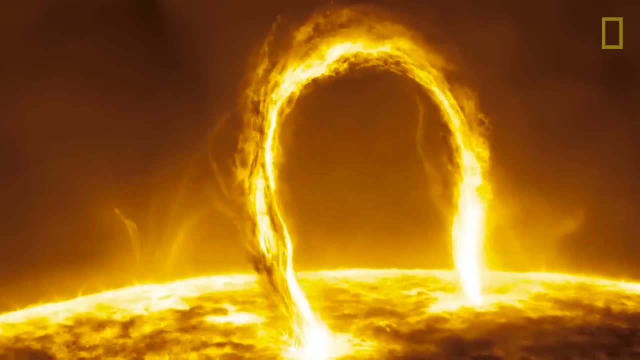 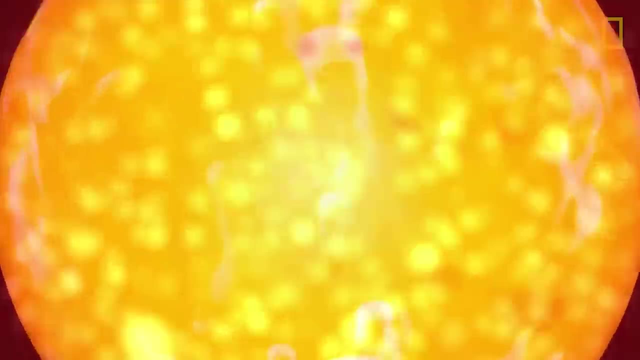 8.9% helium and 0.1% heavier elements such as carbon and nitrogen. Due to the Sun's extreme temperatures, these elements stay in a gas-like phase called plasma In the core temperatures reaching at least 27 million degrees Fahrenheit. 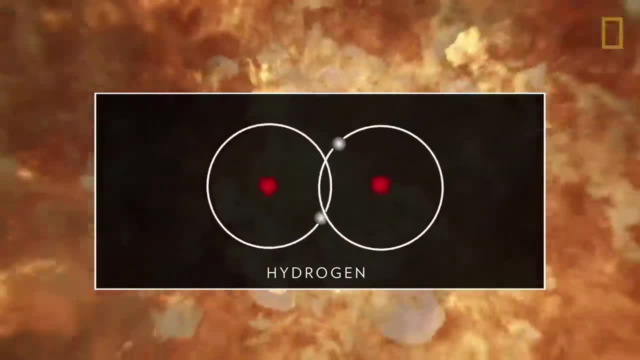 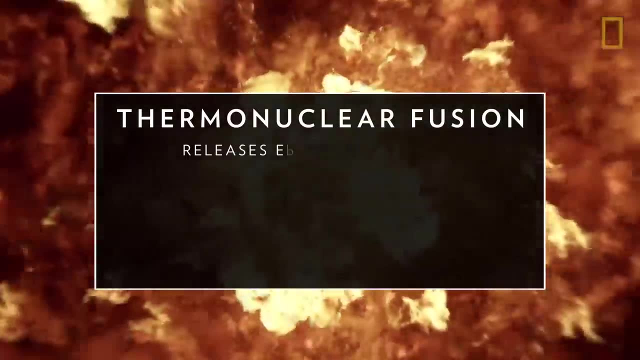 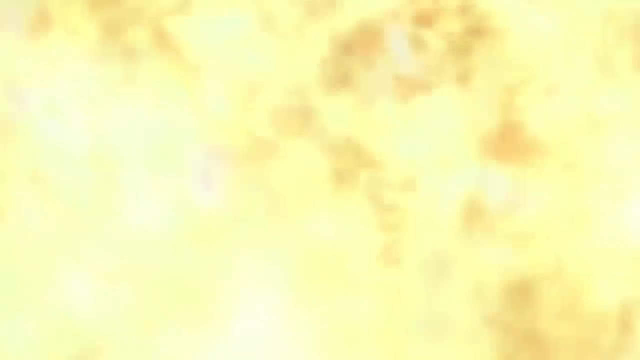 combined with the Sun's powerful energy, can create an enormous amount of energy. This is called thermonuclear fusion, which is a process in which all gravity fuses together hydrogen molecules to create helium, Called thermonuclear fusion. this releases an enormous amount of energy. 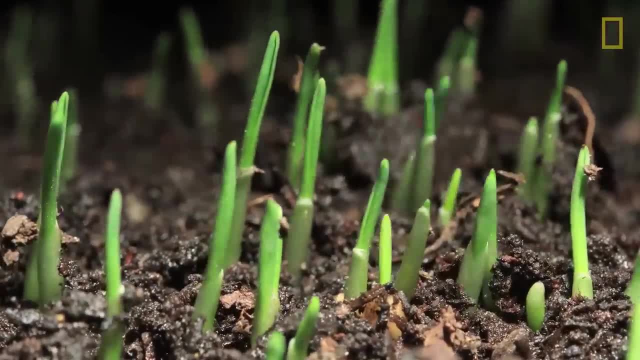 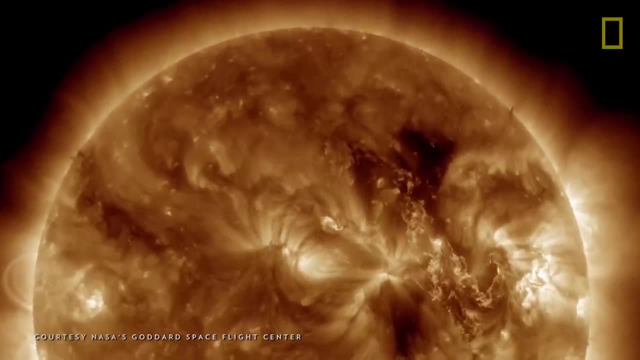 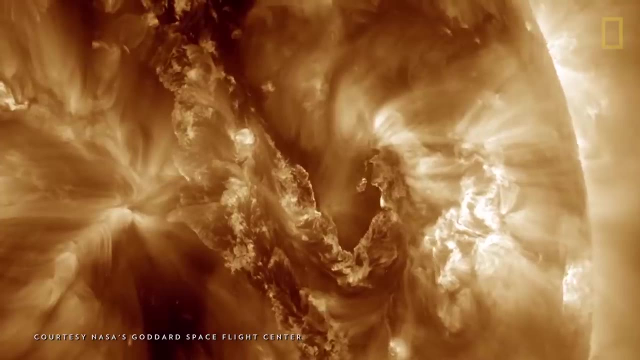 in the form of radiation, electricity, solar wind and, as we experience on Earth, life-giving heat and light, Thanks to the Sun's tremendous gravity. it's strong enough to hold the solar system intact and is primarily due to the Sun's size and mass. 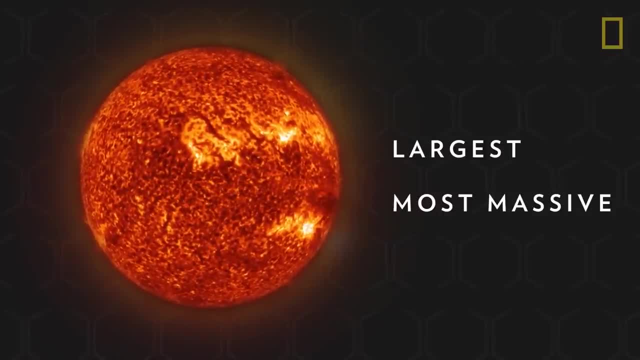 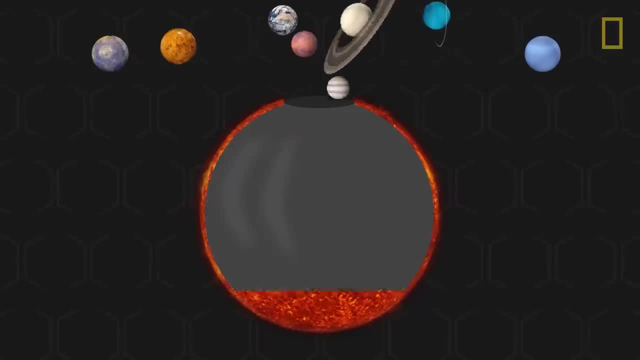 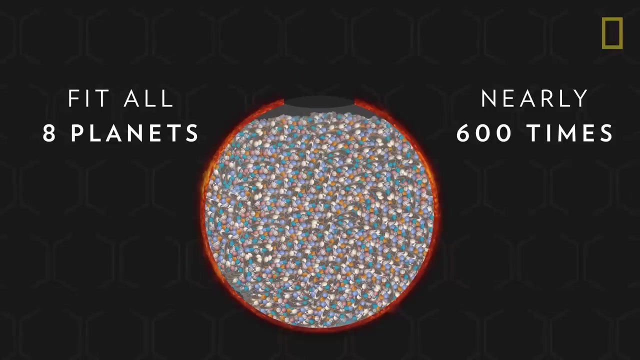 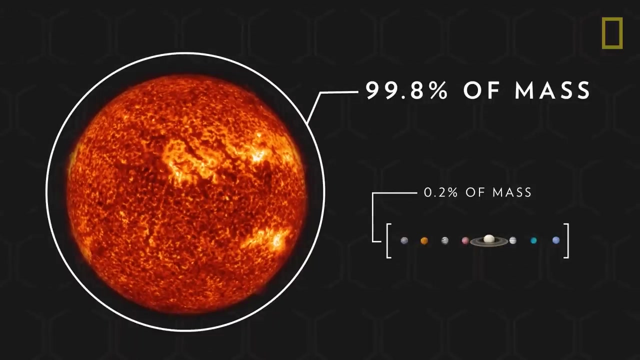 Our Sun is the largest and most massive object in the solar system. It's more than 100 Earths wide and could theoretically fit all eight planets inside nearly 600 times. It also contains approximately 99.8% of all the mass in the solar system. 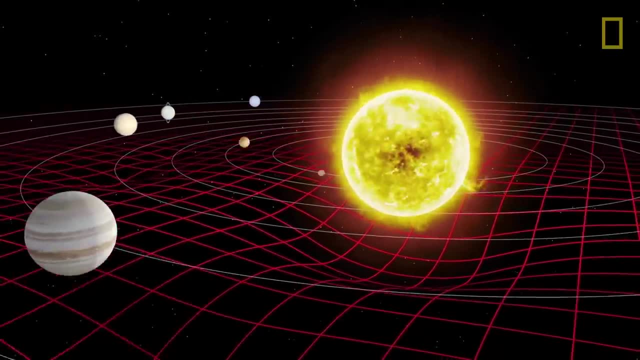 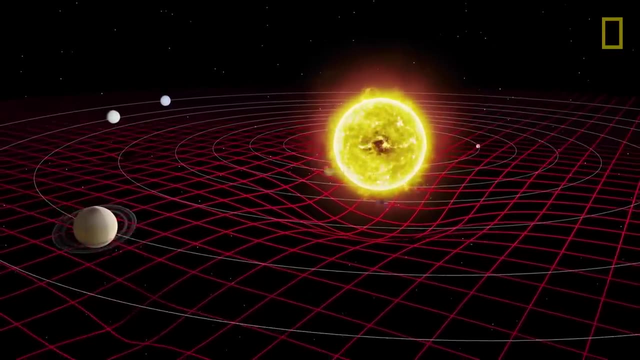 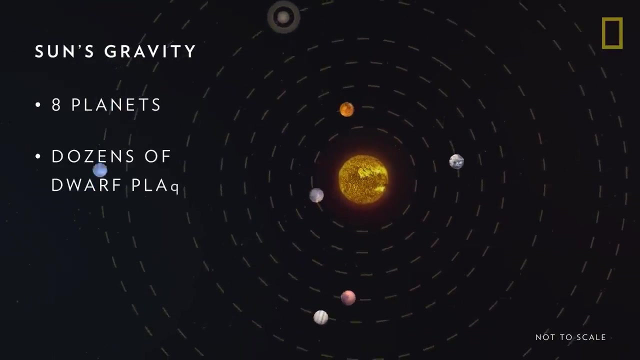 Because of this mass, the Sun has a great pull on the fabric of space, creating a gravitational force that causes nearby planetary bodies to be drawn toward it. This gravitational pull allows the Sun to hold together a system of eight planets, potentially dozens of dwarf planets.